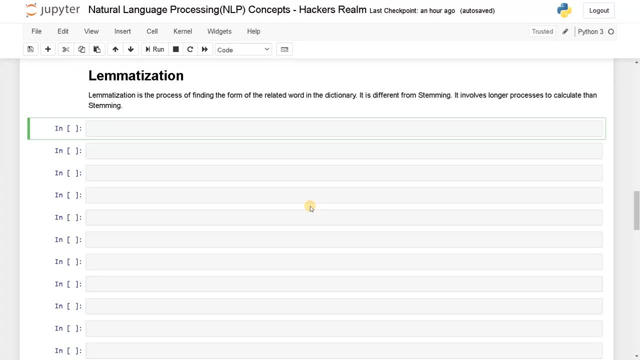 Hey guys, this is Ashwin here In this video we're going to see about lemmatization. So lemmatization is the process of finding a form of the related word in the dictionary. So it is completely different from stemming. It will also try to find the root of the word but that particular word. 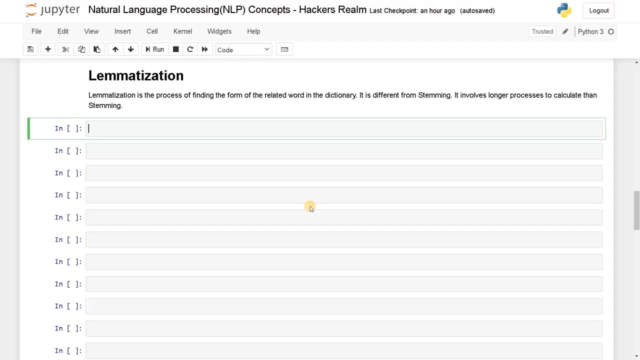 will be present in the dictionary. So that is the only difference between lemmatization and stemming, And it also involves some longer processes because of the algorithm. So this will give us some meaningful words and like stemming. So let's see how it works First. 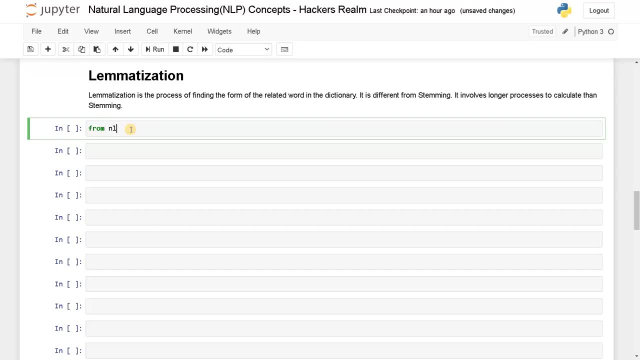 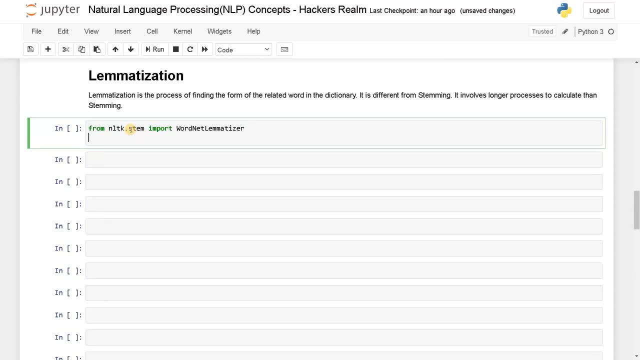 I'm going to import the module from nltkstem, import WordNet lemmatizer. So I will say lemmatizer, lemmatizer equals WordNet lemmatizer, run this. So let's convert a few words and see how it's working. So lemmatizer dot lemmatize Here, I'll just pass. 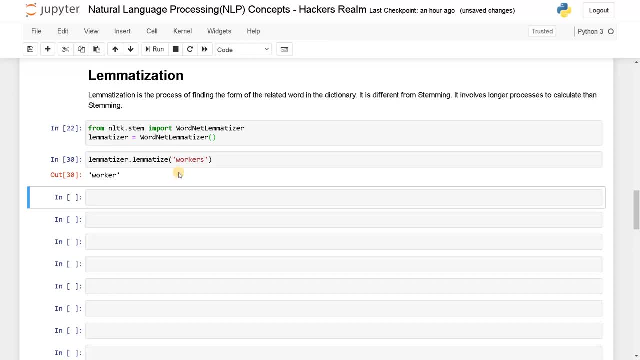 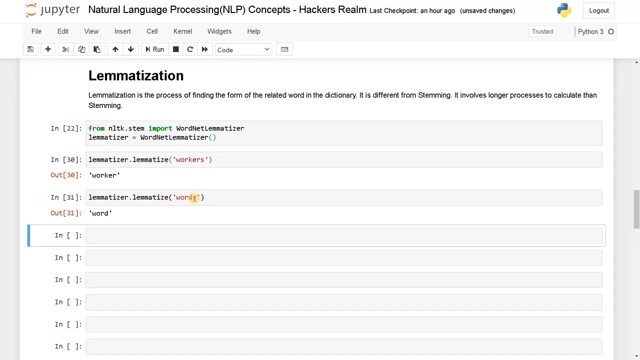 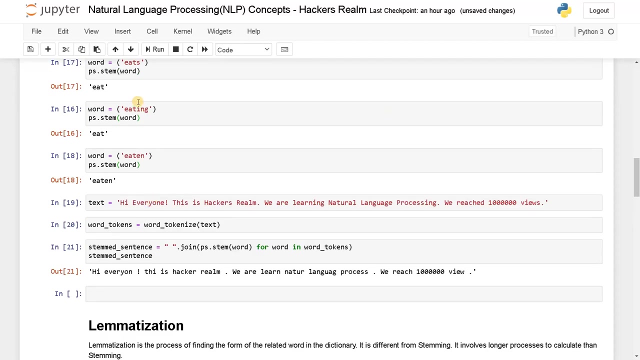 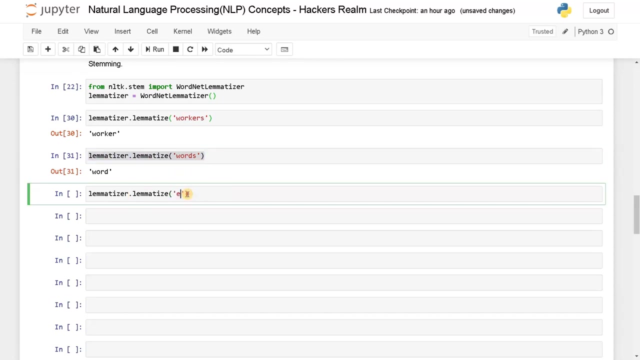 workers. So here you can see. you just remove the word Yes and gave us a worker. Let's see for another word, Words. So let's change the overview. So workers, From this each just giving the whole thing Eats, because we've also done it in the stemming. So it's from this eats, just giving the whole thing. 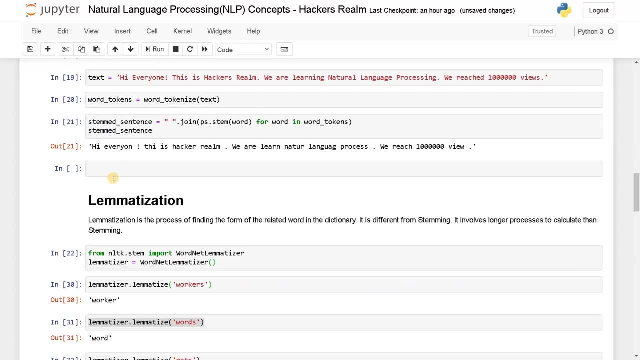 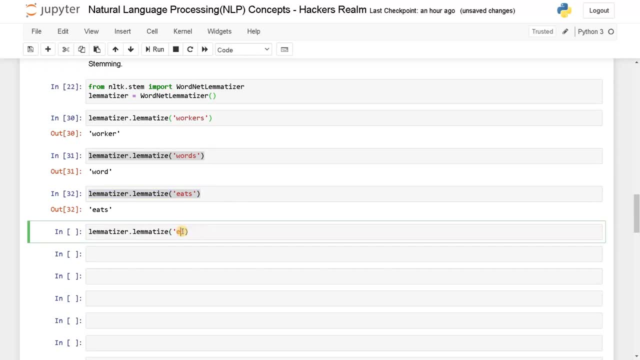 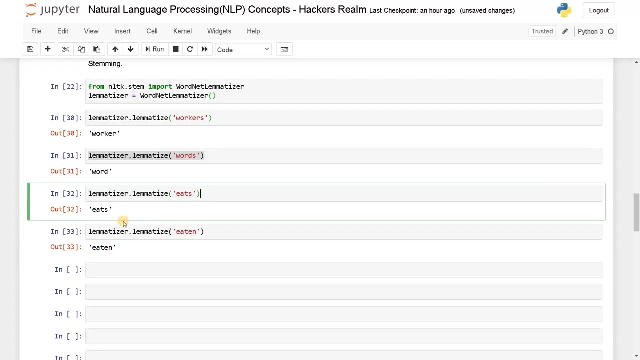 whole thing. so in the stemming it just reduced to eat and even if you take like a different word, so i'll just say eaten. so here also just saying eaten. um, so some words. uh, it's not able to truncate because of the algorithm, so you just need to uh get the word that is present. 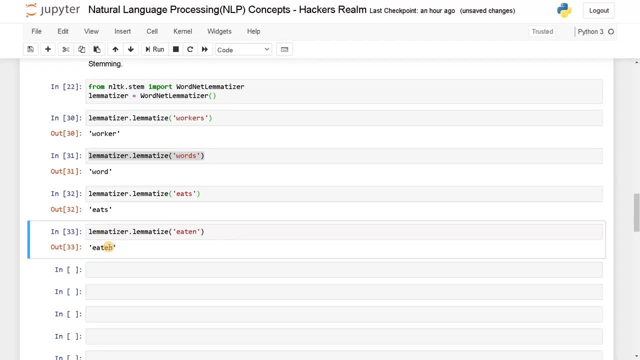 in the dictionary, so e10 will be present in the dictionary. that's why i just uh, going for this, and most of the time it is just removing the additional plural word in order to get the word that is present in the dictionary. so let's try another word called 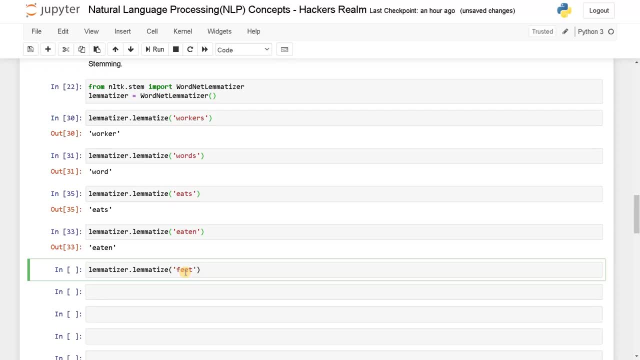 feet. so this is just like a plural form of foot. so run this, see it. just change the word to foot. it's actually giving us like a singular form that the words are present in the dictionary. one more example: maybe i'll just remove these things because it didn't give us the results. 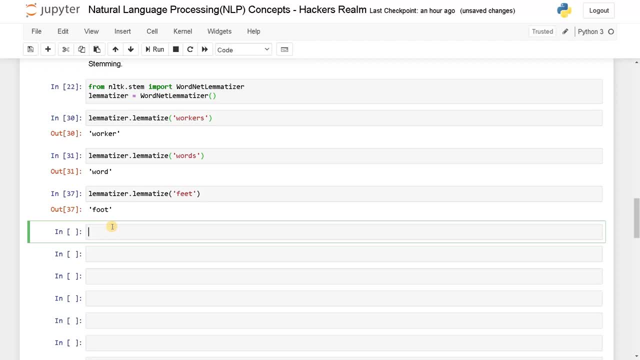 now we can also add some parts of speech. we will see that in the next video. so, using the parts of speech, we can able to clearly, uh, do the lemmatization. so just paste this, and here i will call this as stripes. so stripes, if i consider this as a verb. 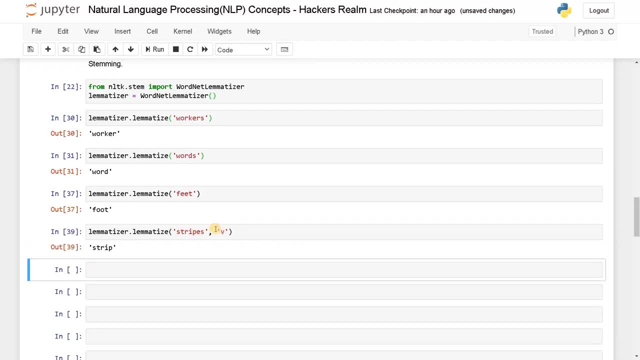 okay, this is stripes, so if i consider this as a verb, it just giving a strip. so let's consider this as a noun, so n and this it's giving us a stripe. so, based on the parts of speech, uh, it is actually giving us a better results, uh, compared to what we have before. so it's better to use the parts of speech and get. 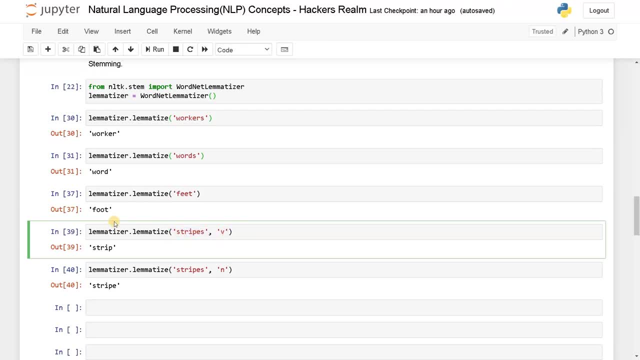 the output like this, and after that we can use the parts of speech and get the output like this, and after that pass the words in into the lemmatization process. so it's actually giving us like a root word that is present in the dictionary. so, based on the verb or noun, it's actually giving us the result. 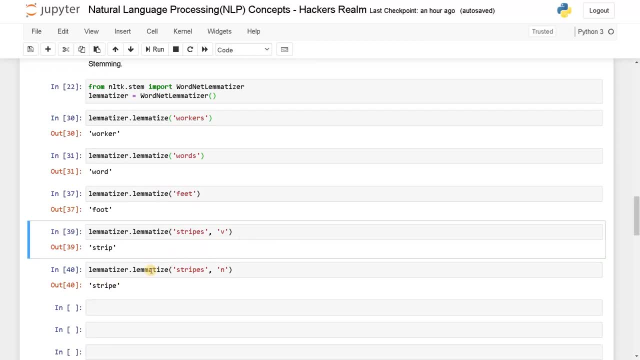 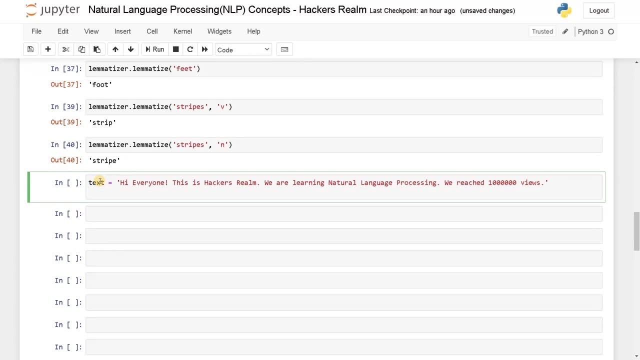 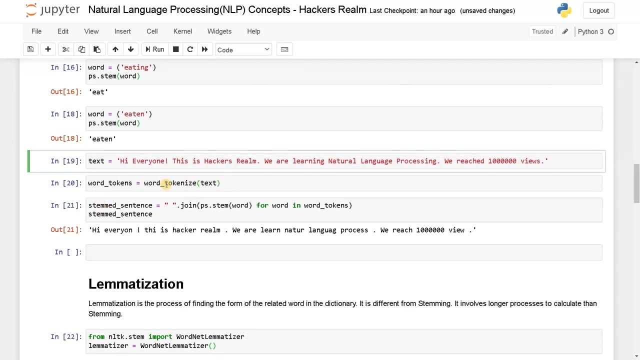 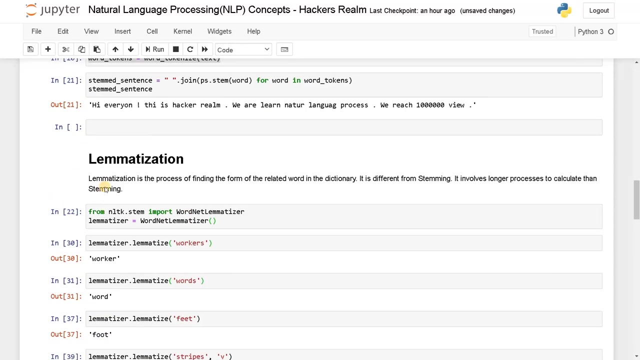 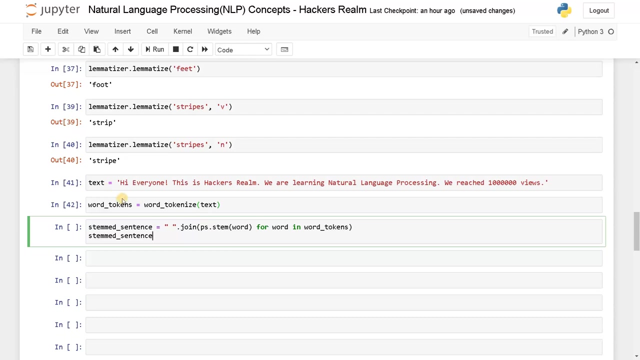 now let's do the same process, what we have done for the stemming. we will take the text here and this, and we will just take the tokenized sentence. so word tokenize, run this and finally we will be getting the lemmatized sentence. so here i'll just pass lemmatizer, dot, lemmatize here, and this will be lemmatized sentence. 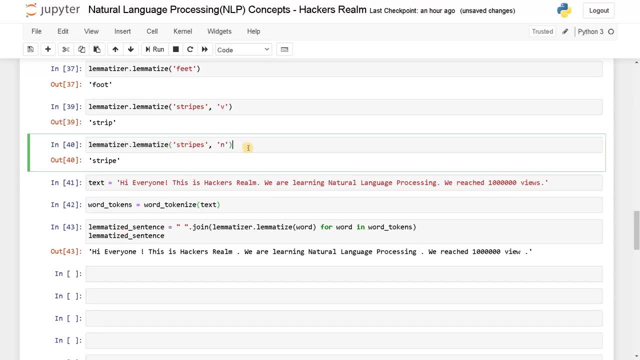 okay, run this now here. it didn't uh remove. uh, i think it didn't remove anything, as you can able to see. hi everyone, this is hackers realm. uh, we are learning natural language processing. uh, we reached, uh, one million views. okay, only this. views has been changed to.